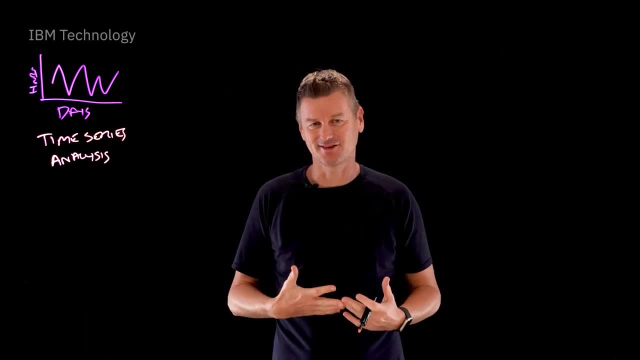 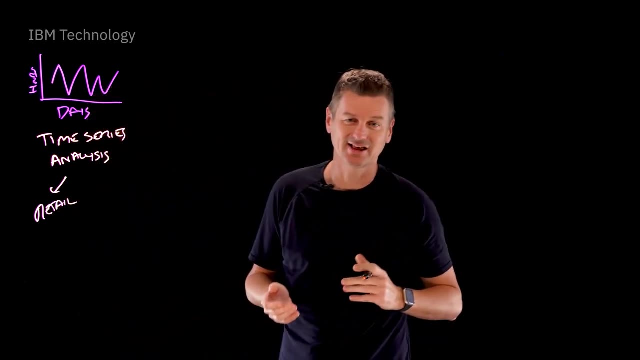 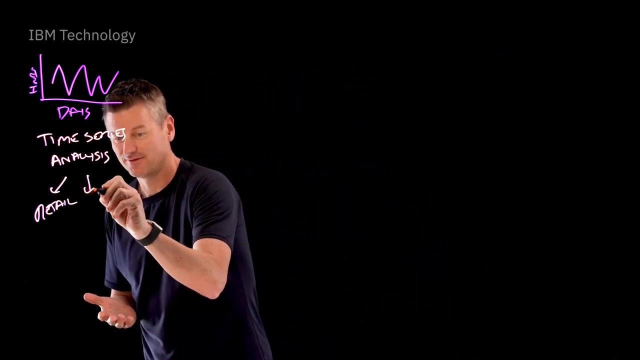 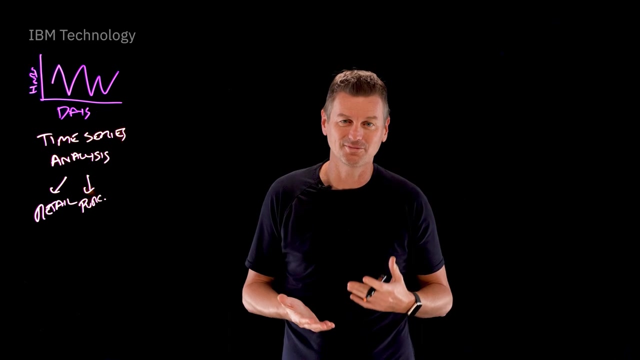 organisations drive better business decisions. So, for example, using time series analysis, a retailer can use this functionality to predict future sales and optimise their inventory levels. Conversely, if you're into purchasing, a purchaser can use time series analysis to predict commodity prices and make informed purchasing decisions. 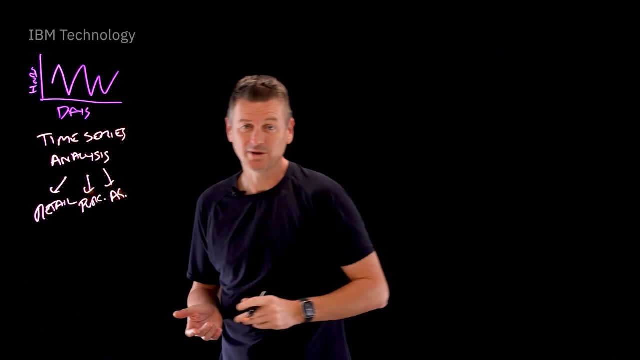 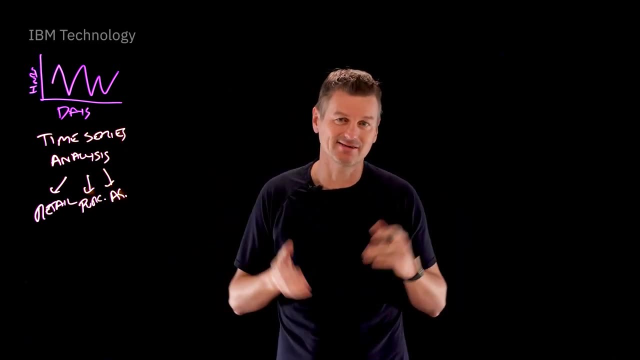 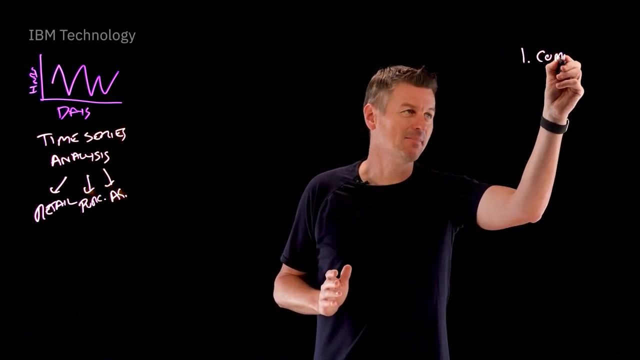 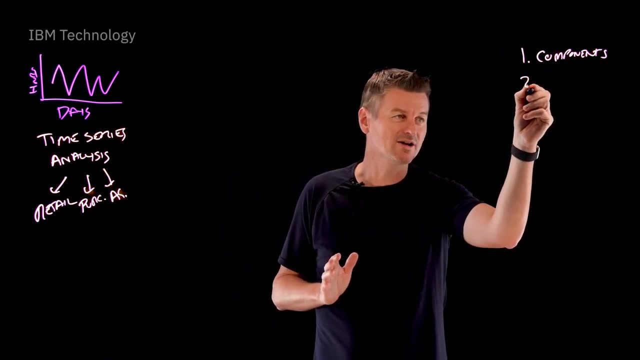 And then, in fields like agriculture, we can use time series analysis to predict weather patterns influencing decisions on harvesting and when to plant. So let's first of all introduce number one, The components of time series analysis, and then number two- we're going to take a look. 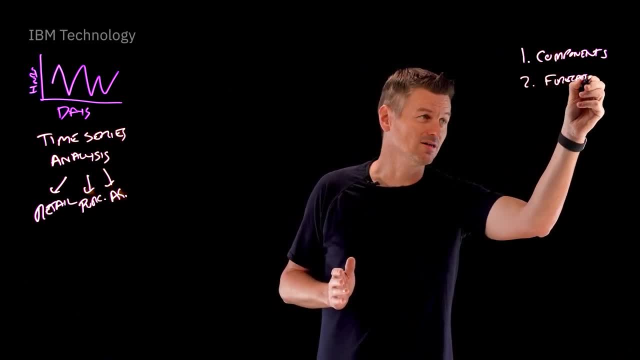 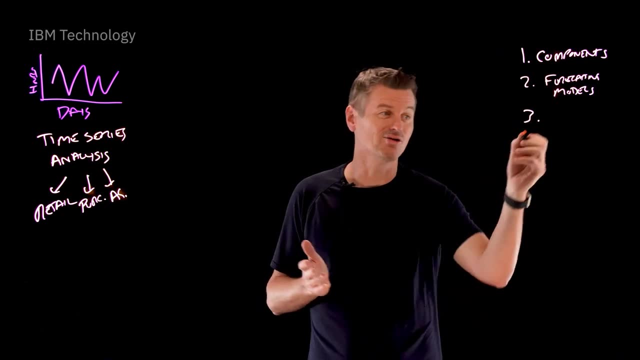 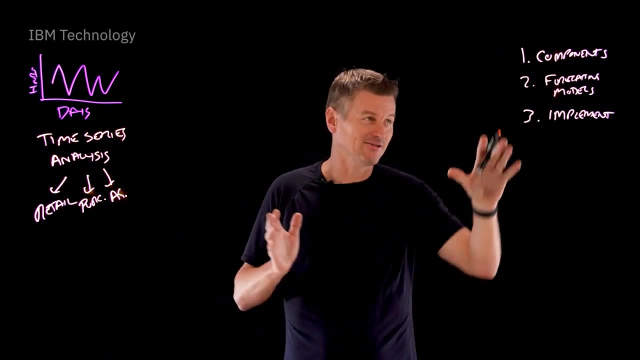 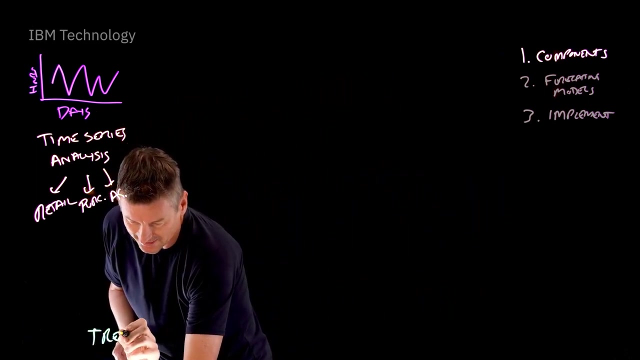 at some of the forecasting models for performing time series analysis. And then, number three, we're going to talk about how to implement some of this stuff. OK, now let's talk about the components first of all, And one component is called trend. 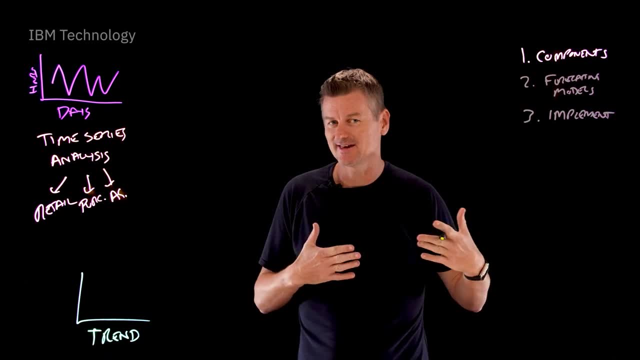 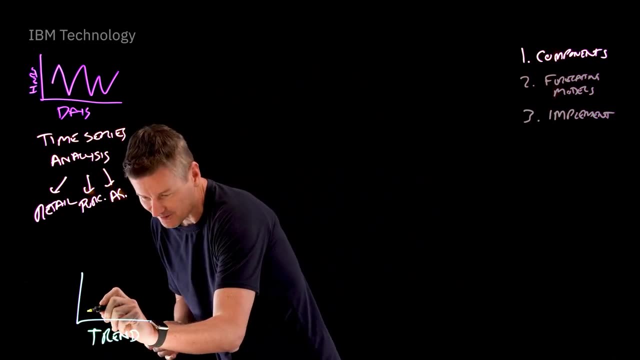 Now, this component refers to the overall direction of the data over time, whether it's increasing, whether it's decreasing, perhaps it's staying the same, So you can think of it like a line on the graph that's either going up or going down. 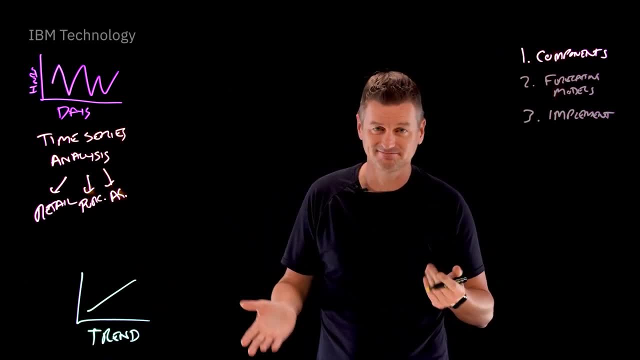 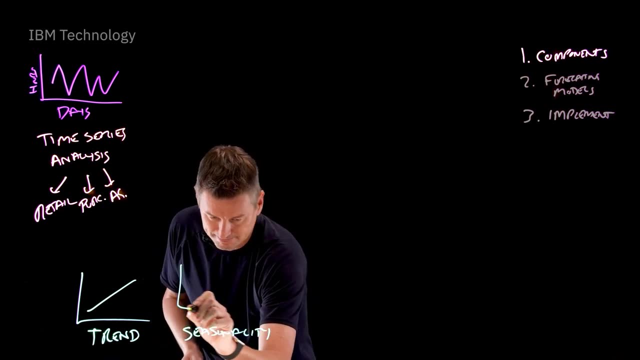 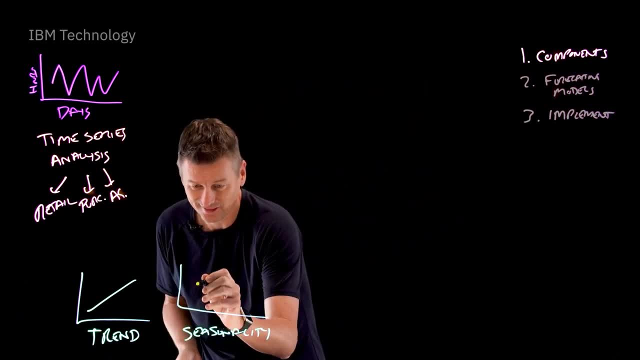 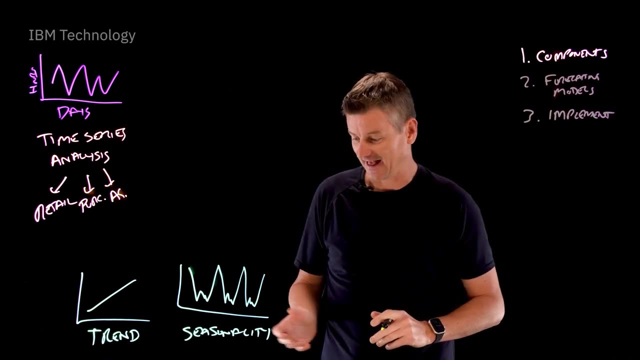 way that retail sales spike during the holiday season, So we might see a spike and then a bit lower. The spike is back and it repeats. like that. That's seasonality. Third component: that's cycle, And cycle refers to repeating but non seasonal pattern. 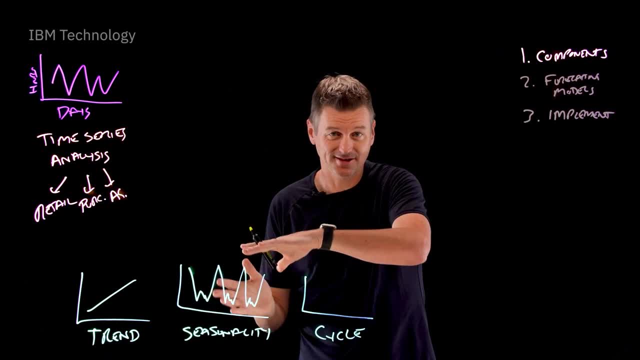 It keeps repeating such pattern over a in-course holiday, becoming theales are working. It means it never stops, So it's really a cycle. even it has not a cycle, So it always keeps repeating patterns in the data. So these might be economic booms and busts that happen over several years. 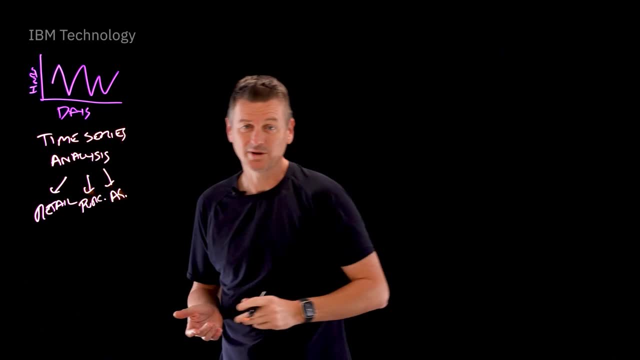 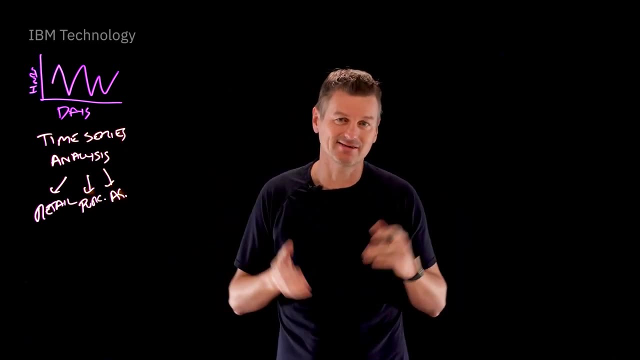 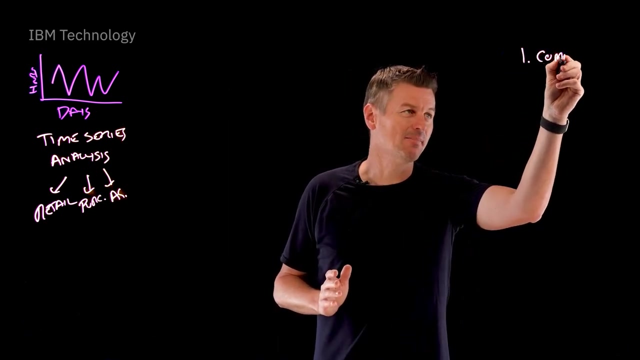 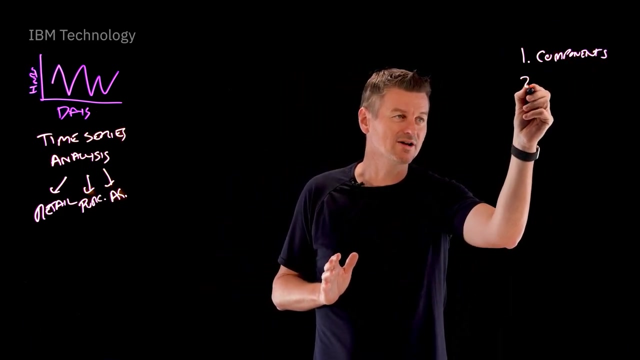 And then, in fields like agriculture, we can use time series analysis to predict weather patterns influencing decisions on harvesting and when to plant. So let's first of all introduce number one, The components of time series analysis, and then number two- we're going to take a look. 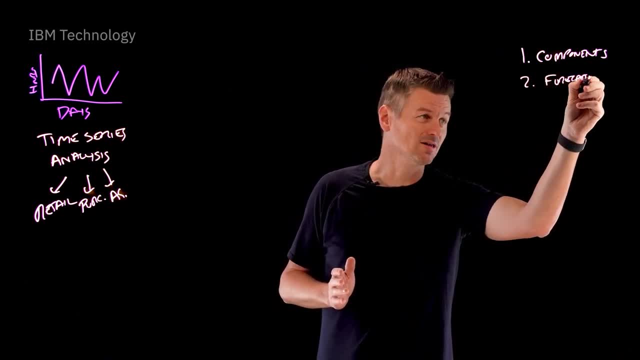 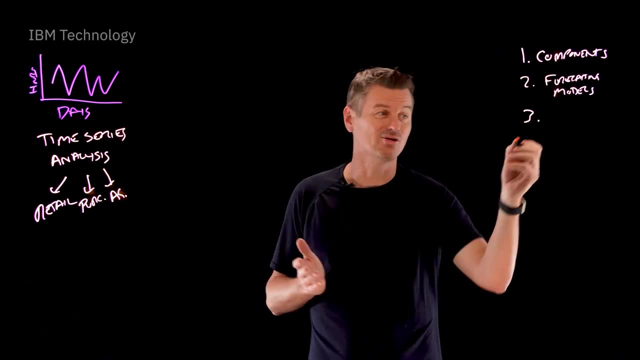 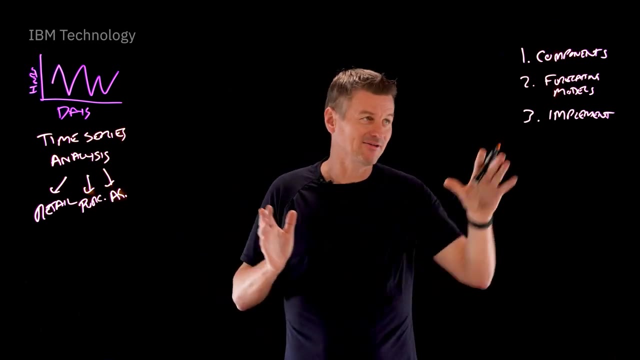 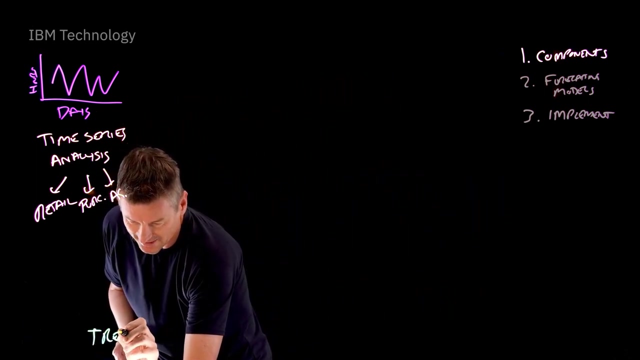 at some of the forecasting models for performing time series analysis. And then, number three, we're going to talk about how to implement some of this stuff. OK, now let's talk about the components, first of all, And, And. one component is called trend. 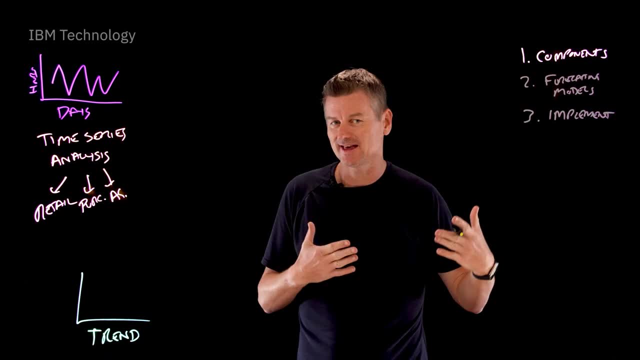 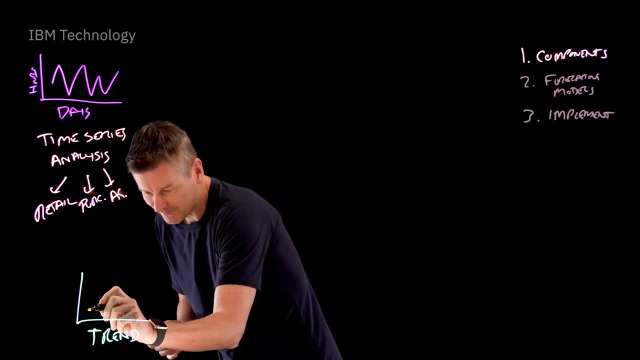 Now, this component refers to the overall direction of the data over time, whether it's increasing, whether it's decreasing, perhaps it's staying the same. So you can think of it like a line on the graph that's either going up or going down, or 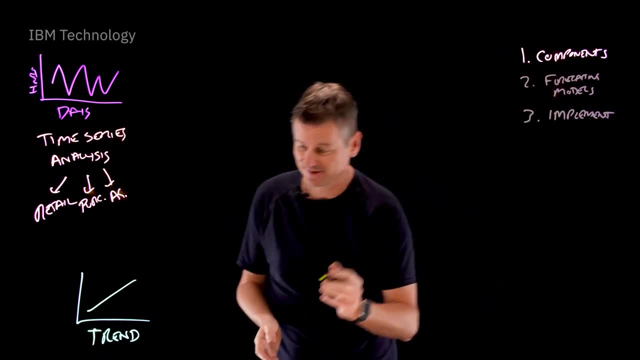 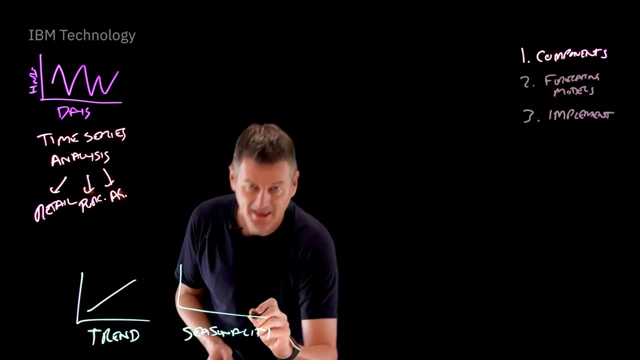 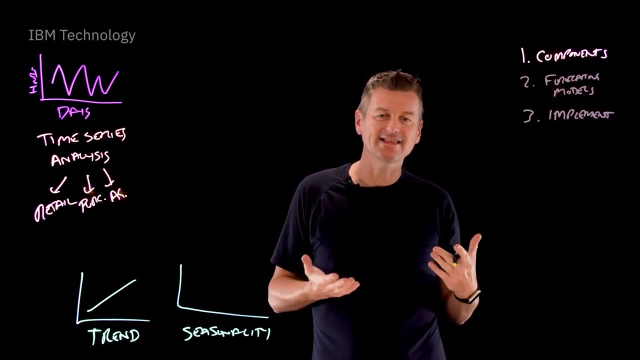 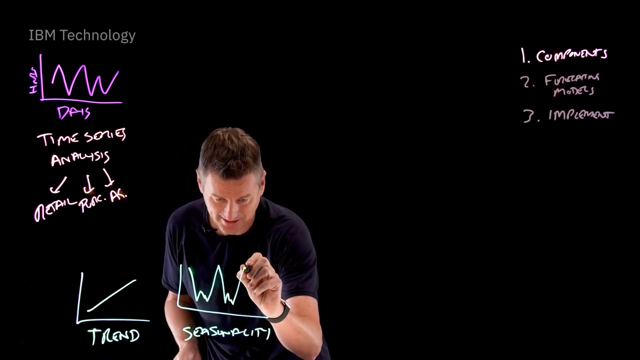 staying flat. That's the first component. The second one, seasonality. Now, this component is a repeating pattern of data over a set period of time, like the way that retail sales spike during the holiday season. So we might see a spike and then lower. the spike is back and it keeps repeating like that. 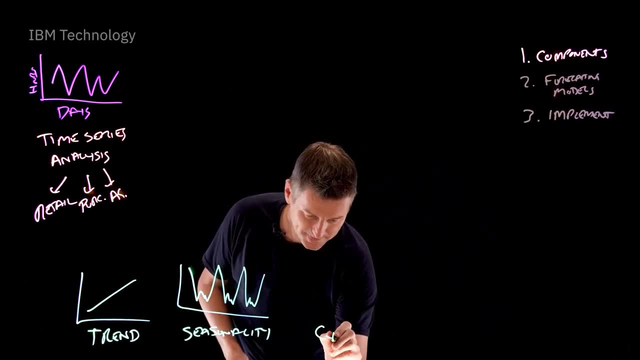 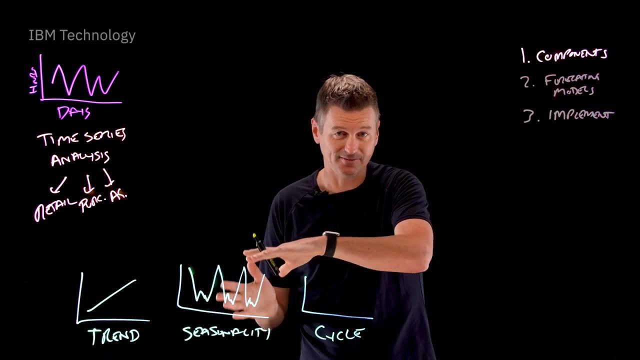 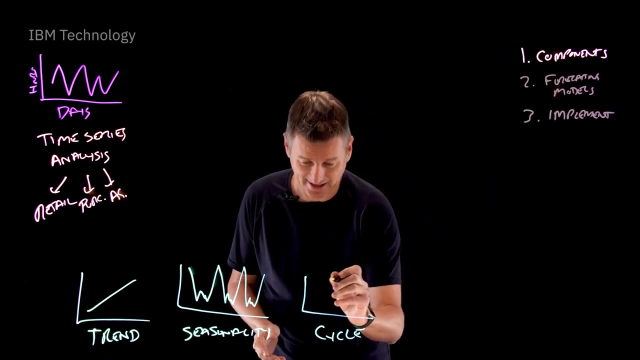 That's seasonality. Third component, that's cycle, And cycle refers to repeating but non-seasonal patterns In the data. So these might be economic booms and busts that happen over several years or maybe even decades. So it's a much smoother curve. 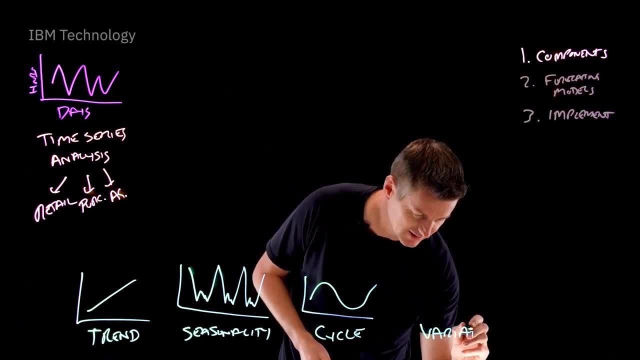 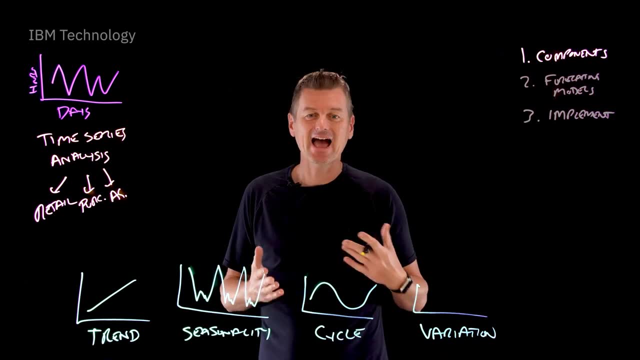 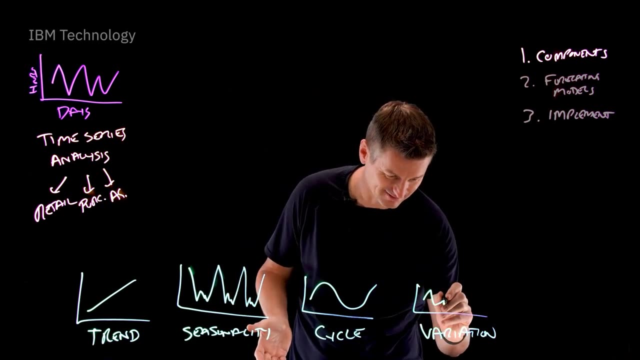 And then, lastly, there is variation, And variation refers to the unpredictable ups and downs in the data that cannot be explained by these other components, And this component is also known as irregularity or noise. And well, it looks like, maybe, that. 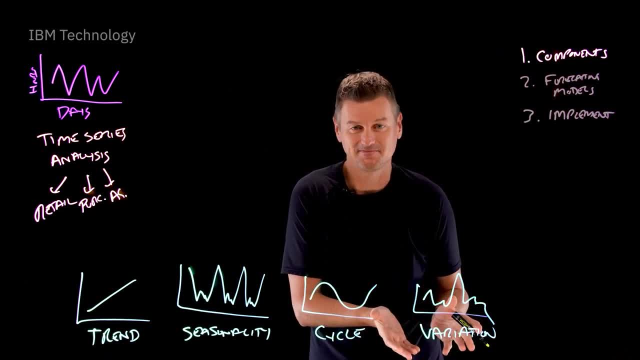 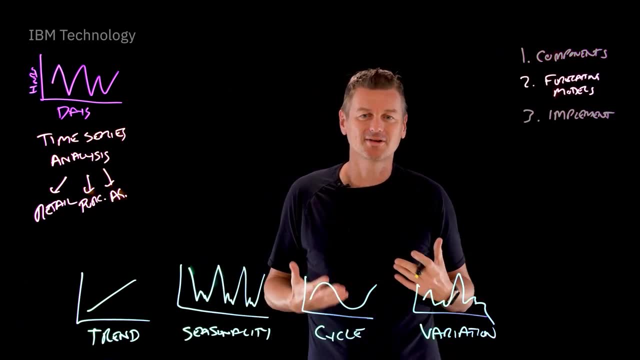 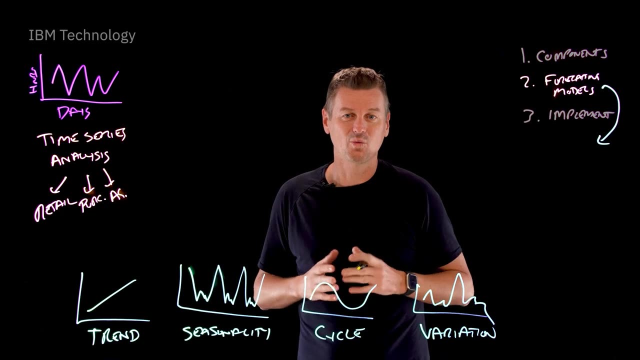 Yeah, very difficult to pick out the trend. So those are some of the components of time series, But let's talk about the forecasting models that we can use to perform some analysis, And there are several popular forecasting models out there. One of the most well known is called the ARIMA model. 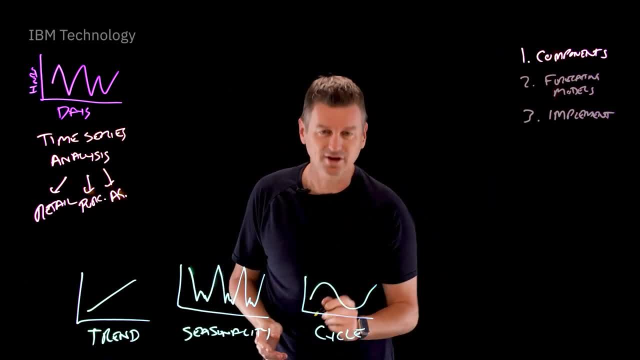 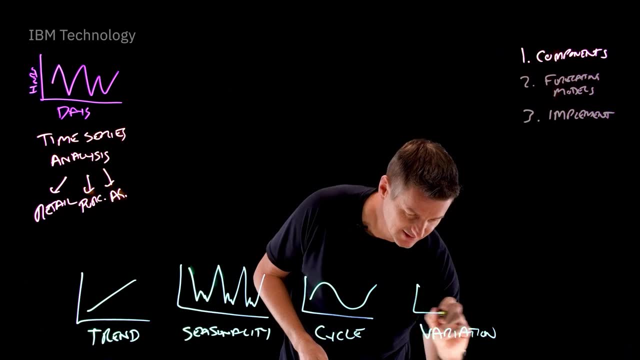 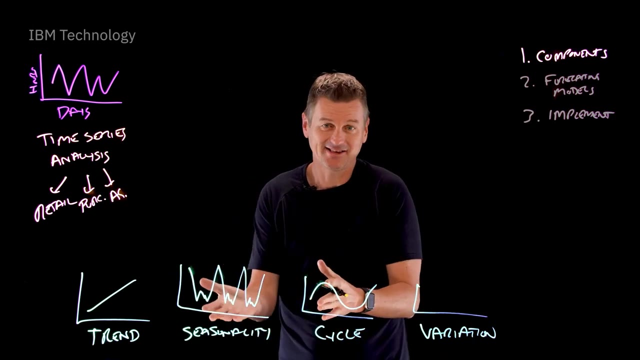 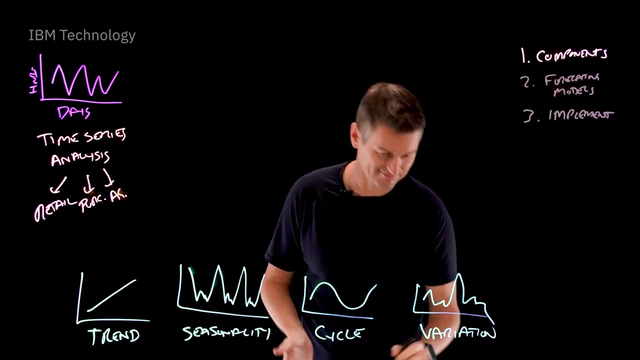 or maybe even decades, So it's a much smoother curve. And then, lastly, there is variation, And variation refers to the unpredictable ups and downs in the data that cannot be explained by these other components, And this component is also known as irregularity or noise. And well, it looks like maybe that, Yeah, very difficult. 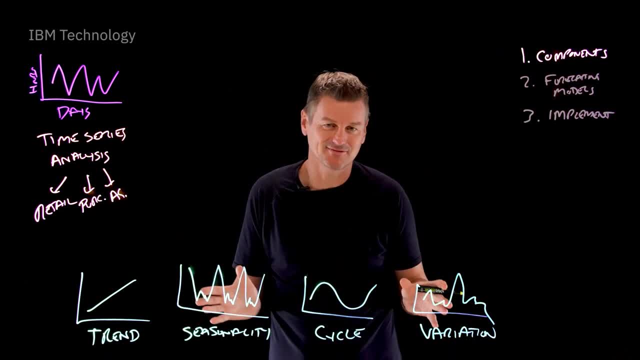 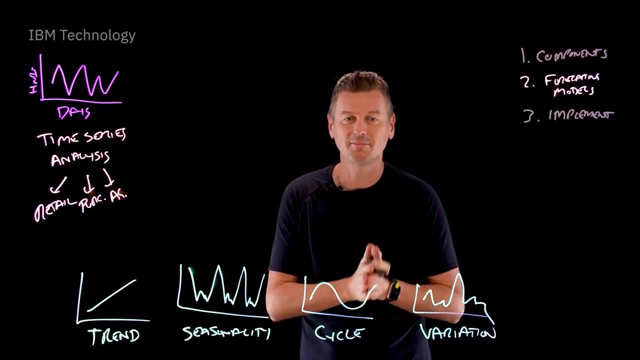 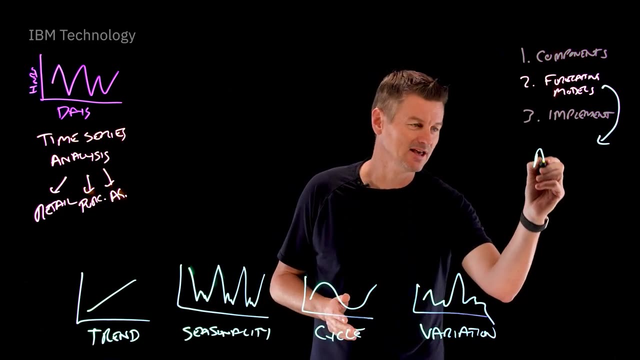 to pick out the trend. So those are some of the components of time series, But let's talk about the forecasting models that we can use to perform some analysis, And there are several popular forecasting models out there. One of the most well known is called the AREMA model. 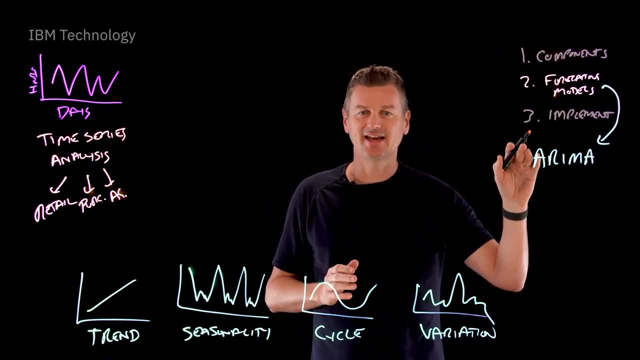 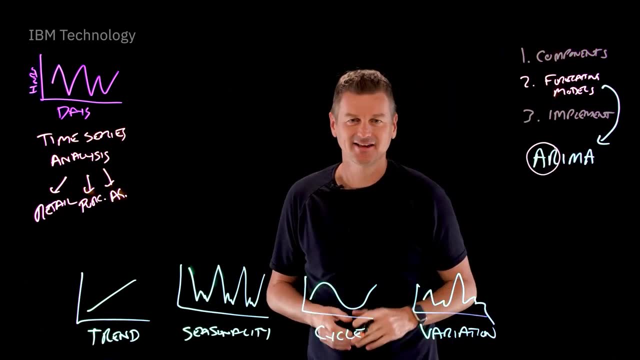 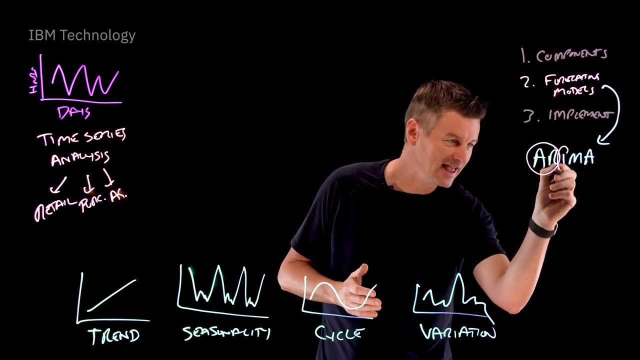 Now AREMA. that stands for Auto Regressive, Integrated Moving Average, And the model is made up of three components. So there's the AR part, That's the auto regressive component And that looks at how past values affect future values. Then there's the I for integrated, 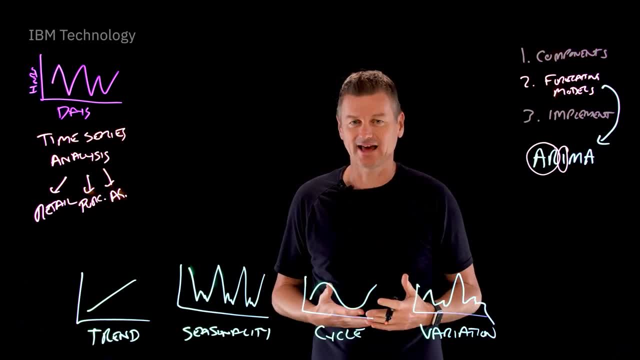 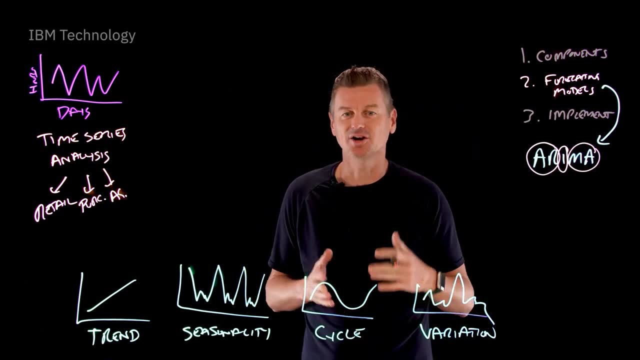 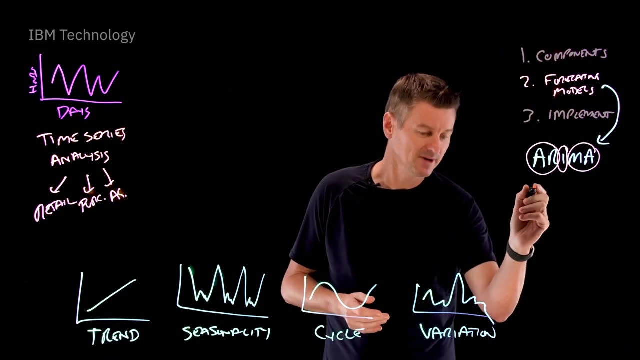 or differencing component, And that accounts for trends and seasonality. And then there is the MA component, That's the moving average component And that smooths out the noise by removing non-deterministic or random movements from a time series. So that's AREMA, another pretty popular one you'll 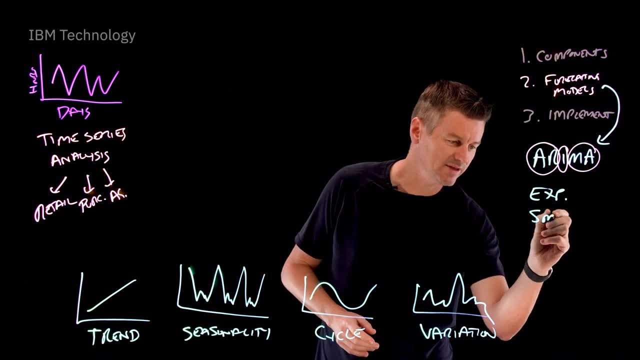 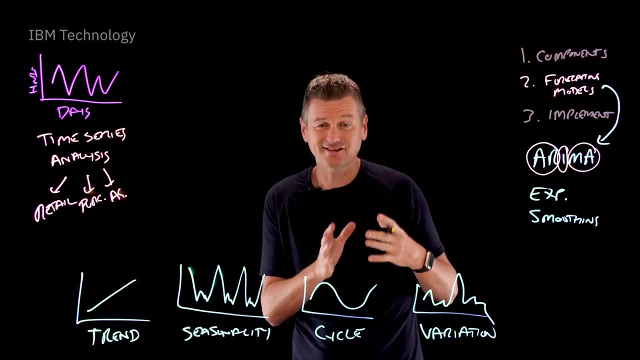 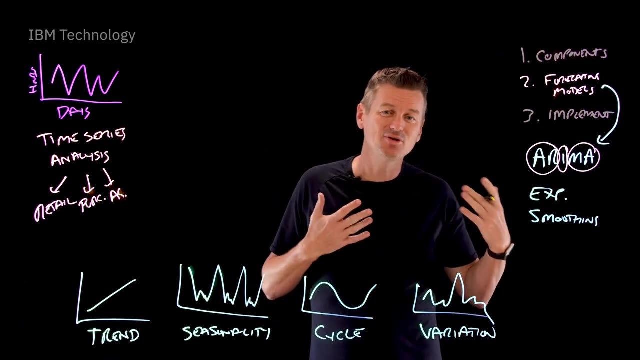 often see is called exponential smoothing, And exponential smoothing is used to forecast time series data that doesn't have a clear trend or seasonality, So it doesn't fit into these kind of areas And this model works by smoothing out the data, by giving more weight. 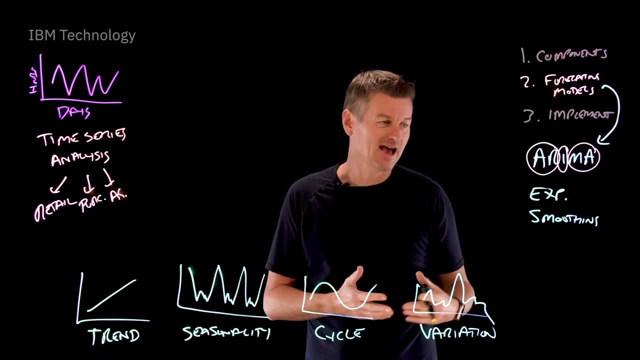 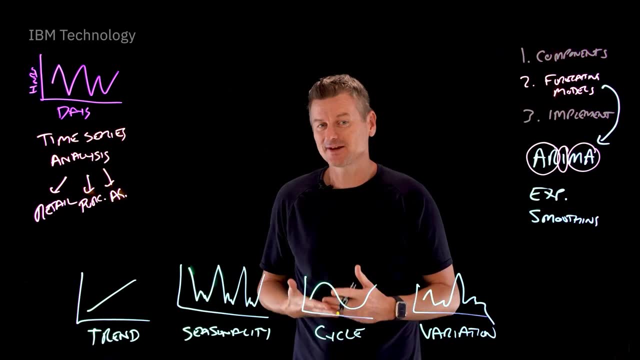 to recent values and less weight to older values. And there are many other forecasting models out there, and the right one to use, of course, depends on the data you're working with and the specific problem you're trying to solve. Okay, so let's finally talk a little bit about implementation. 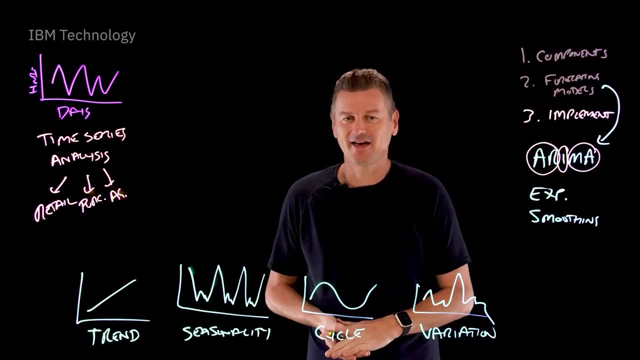 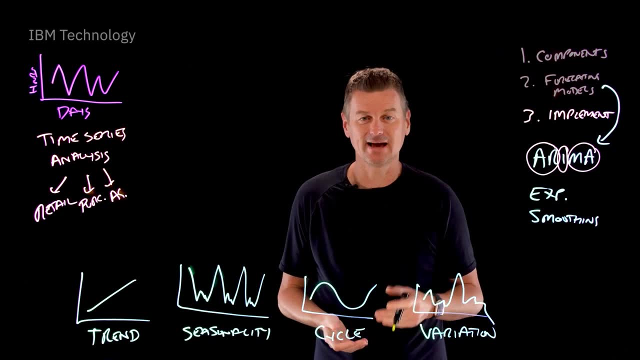 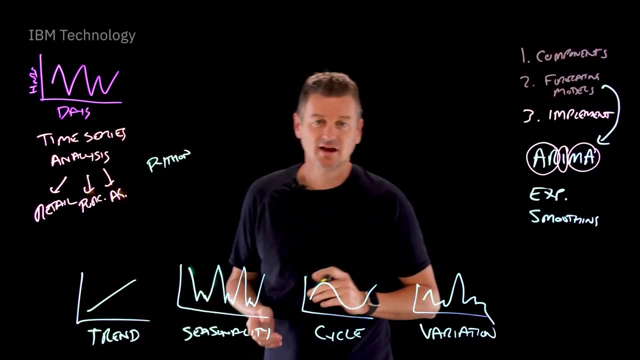 How do we implement this? There are several software packages out there that can help you perform time series analysis and forecasting, such as those with R and Python and MATLAB. So, if we just focus in on Python for a moment, two of the most popular libraries for time series analysis in Python. 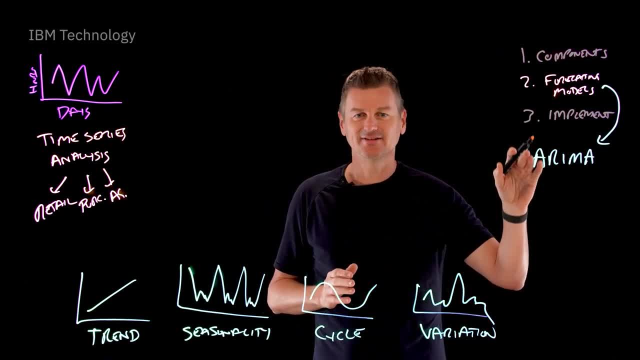 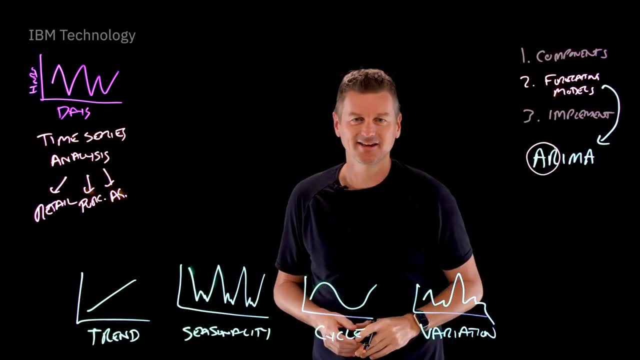 Now ARIMA. that stands for Auto Regressive Integrated Moving Average, And the model is made up of three components. So there's the AR part, that's the autoregressive component and that looks at how past values affect future values. 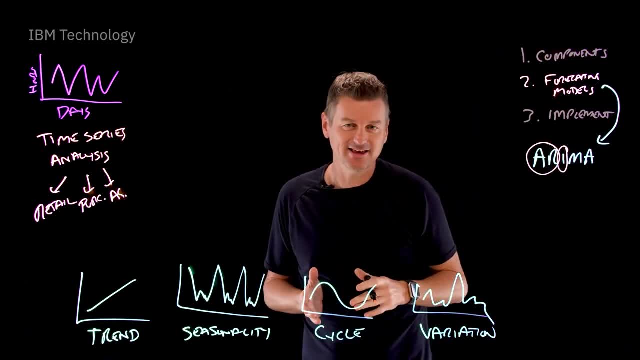 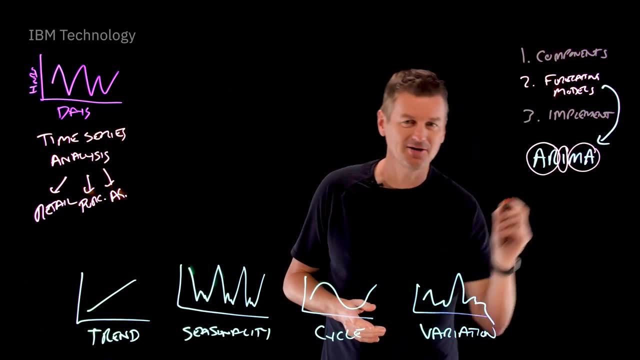 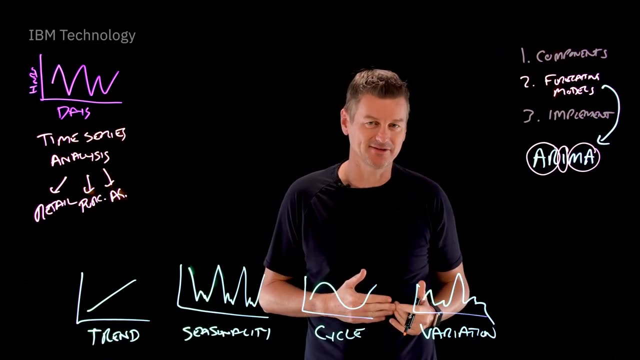 Then there's the I for integrated or differencing component, and that accounts for trends and seasonality. And then there is the MA component, that's the moving average component and that smooths out the noise by removing non-deterministic or random movements from a time series. 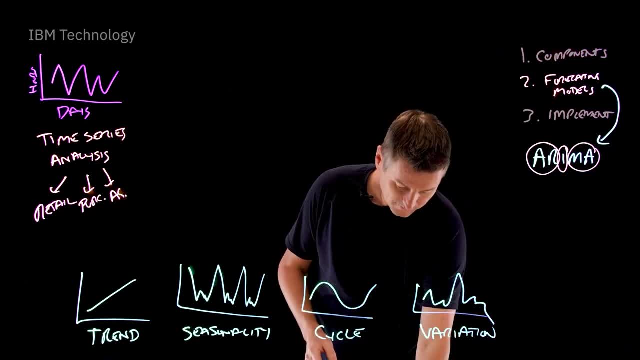 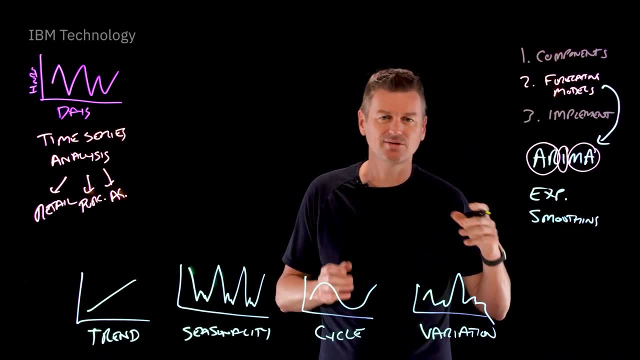 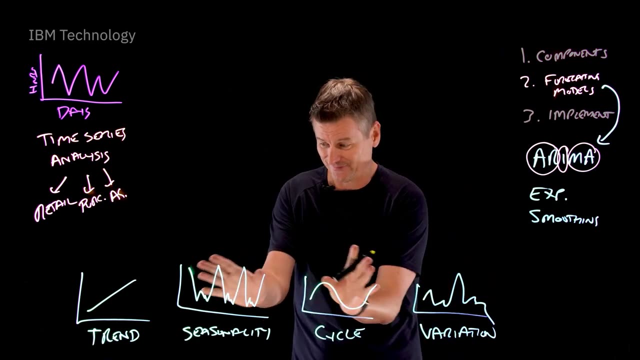 So that's ARIMA. Another pretty popular one you'll often see is called exponential smoothing, And exponential smoothing's model is used to forecast time series data that doesn't have a clear trend or seasonality, So it doesn't fit into these kind of areas. 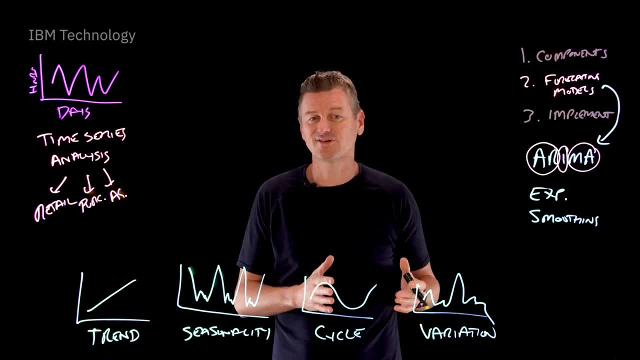 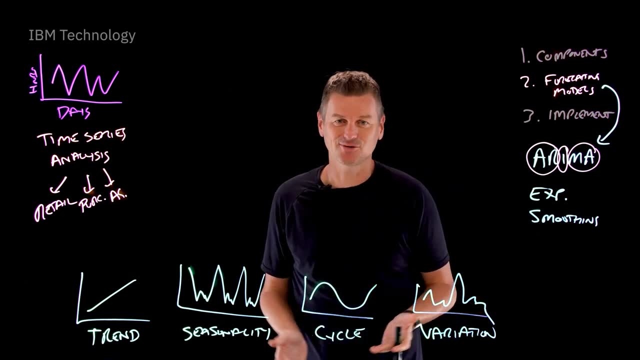 And this model works by smoothing out the data, by giving more weight to recent values and less weight to older values. And there are many other forecasting models out there And the right one to use of course depends- And the right one to use of course depends on the data you're working with and the specific problem you're trying to solve. 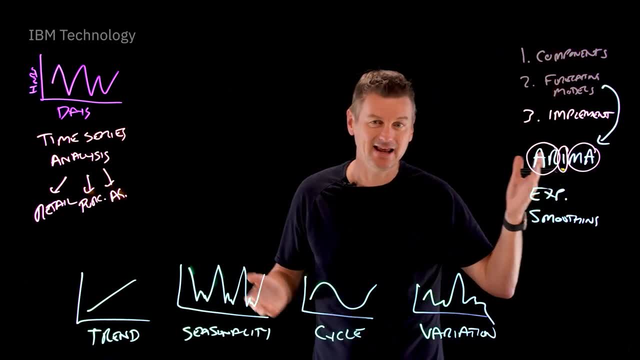 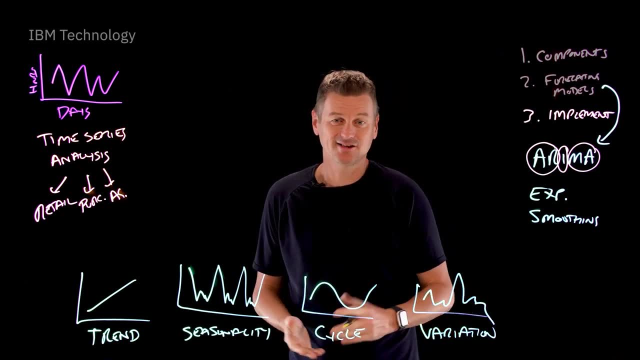 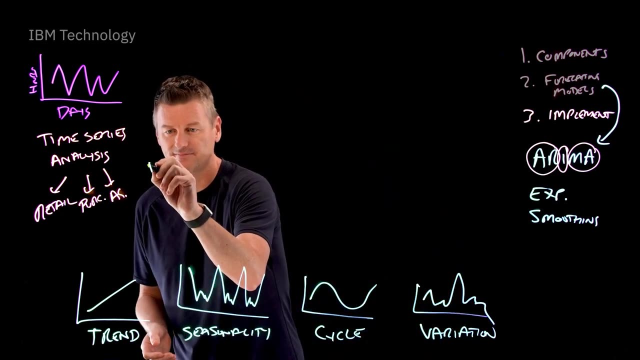 OK, so let's finally talk a little bit about implementation. How do we implement this? There are several software packages out there that can help you perform time series, analysis and forecasting, such as those with R and Python and MATLAB. So if we just focus in on Python for a moment, 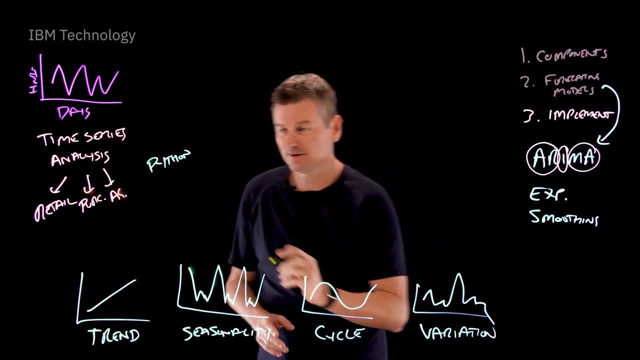 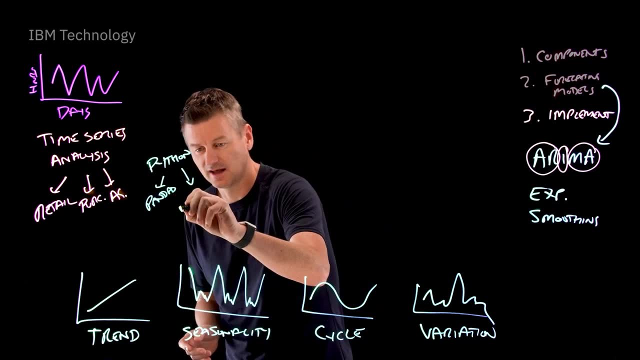 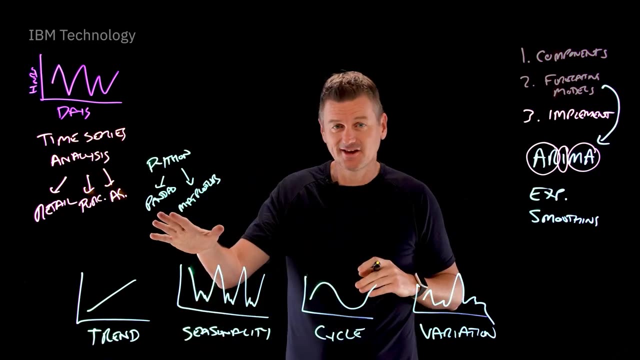 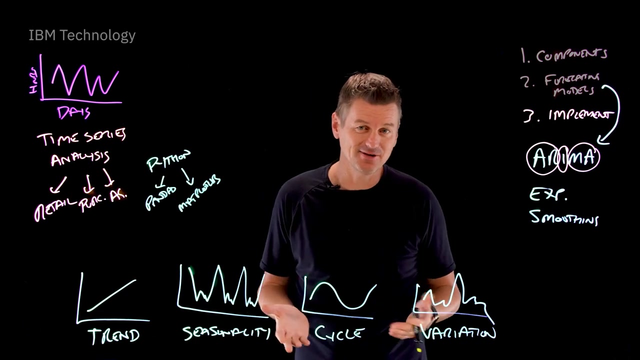 Two of the most popular libraries for time series analysis in Python: Firstly, Pandas, and secondly, a library called Matplotlib. With Pandas, you can easily import, manipulate and analyze the time series data, and it can handle things like missing values, aggregate data and perform statistical analysis on the data. 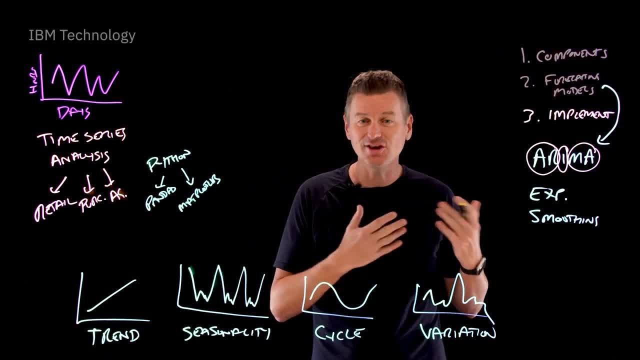 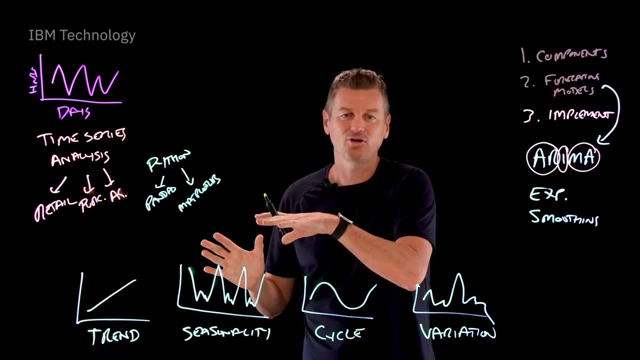 Matplotlib is a library that can help you visualize the time series. You can create line charts or scatter plots and heat maps. Using these libraries, you can perform a wide range of time series analysis tasks like data cleaning, exploratory data analysis and modeling.